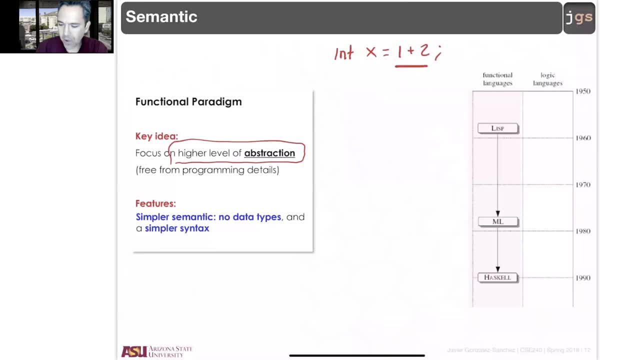 You can ask for one plus two and you can store that in a variable, but there is this idea that you need to define the type of the variable. Moreover, there is this problem that if you do something like division one between two in programming by default in Java, you're going. 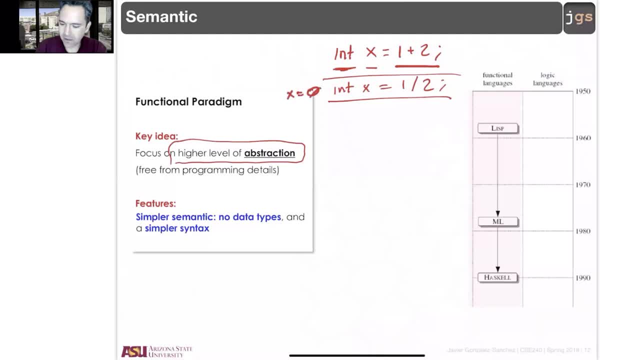 to have this: X equals zero, because you do not define this to be floating point number. So in programming with Java in particular, you are dealing with things like the data types, because Java is not hiding that complexity or those details about type checking from you. 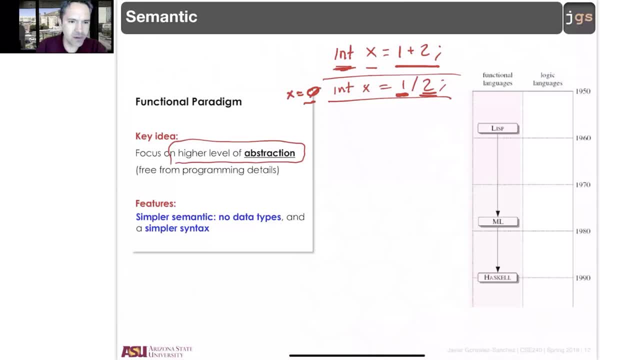 However, if you work in your math class or in your algebra class, the only thing that you get is: I need a variable. That variable is going to be one divided by two, and that's it. And in your math class, you know that this X is going to be 0.5.. You work with numbers and you don't care about. 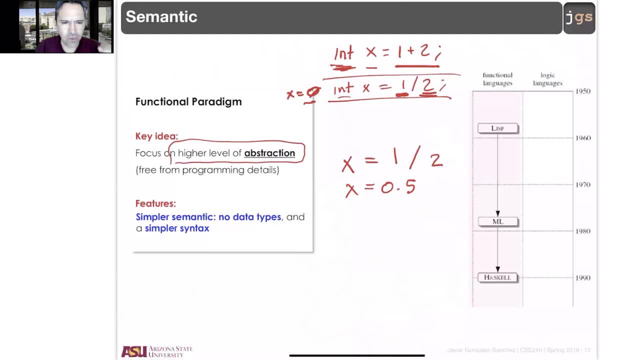 these things about integer, float or so on Math have a higher level of abstraction because in math you don't care about the details about where those numbers are stored. You don't care about those details because the level of abstraction is higher. What Lisp and in general, the functional? 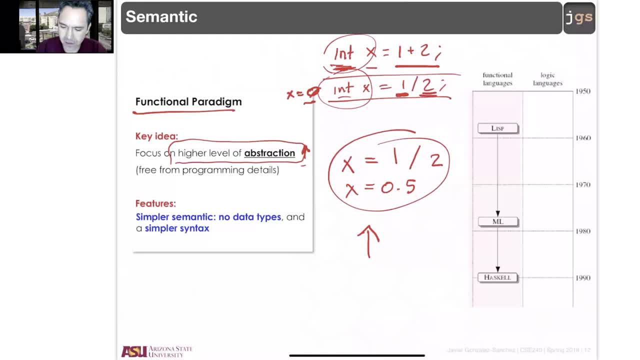 paradigm is is to move abstraction up. That means eliminate these details and make programming look more like math: Focus in the algorithm and forget the details about types, syntaxes and things like that. What do we do? Two things: Semantics and syntaxes. We need to make 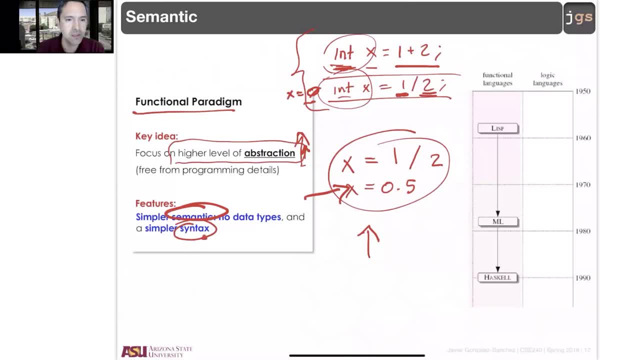 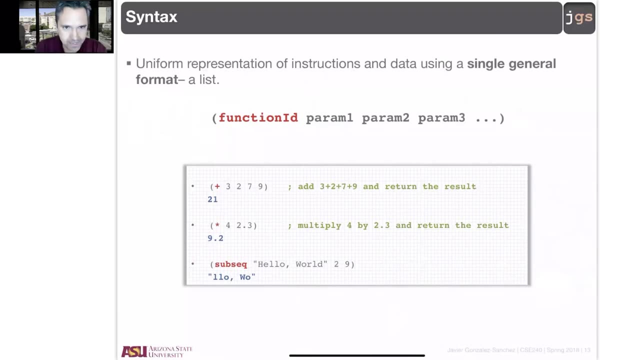 the syntax, all the rules about how to connect words, easy, And we need to make the semantics something that the compiler reviews and fixes, not the programmer. Semantics and syntaxes simpler. Let's see Number one talking about syntaxes In Java, C, C++, something that you need to remember. 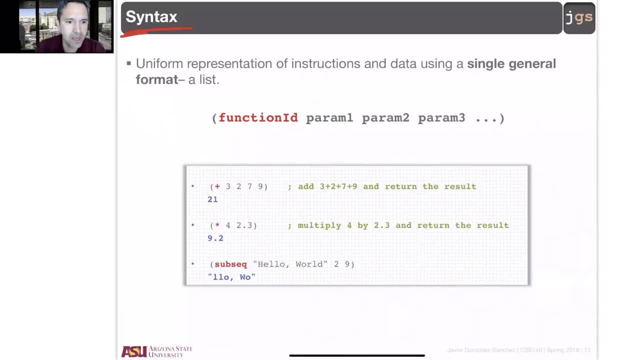 is semicolon. every single line finish and end with a semicolon. Something that you need to remember is curly brackets. Methods have curly brackets. Classes- if you are working with object-oriented programming- have curly brackets. Arrays have square brackets- All of that curly. 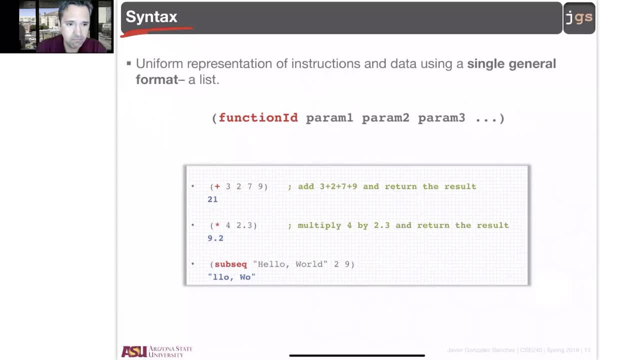 brackets, square brackets, semicolon and so on do not exist in Lisp. The only rule for the syntaxes in Lisp is the following: Number one or 1.1, everything, every instruction, whatever you want to do, starts with a parenthesis and ends. 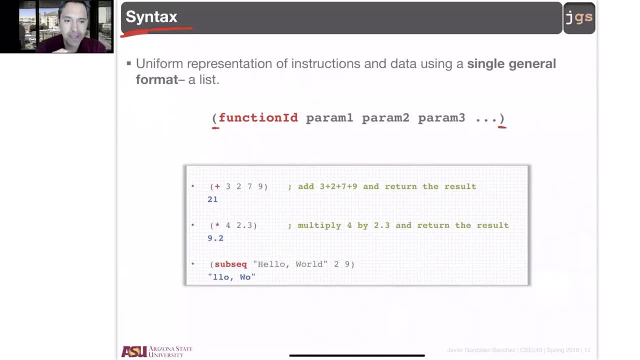 with a parenthesis. Second, any action that you want to do, any instruction, any operator, any method, anything that do something in a program is called a function, Function, Anything. There is no operators, There are functions. There are no methods, There are functions. There are no instructions, They are. 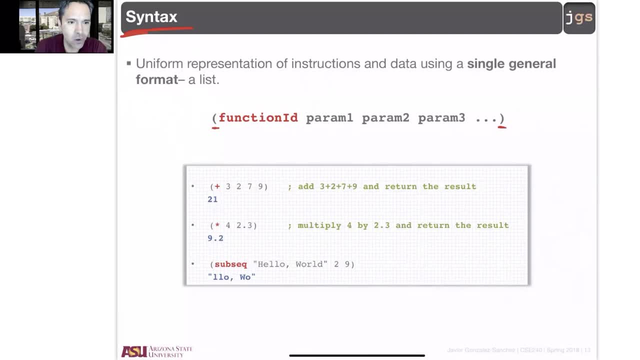 functions. Function is the name for anything that do an action, anything that provide a result. Syntactical rule: The name of the function always, always, always is the first thing inside of the parenthesis. So you open a parenthesis. 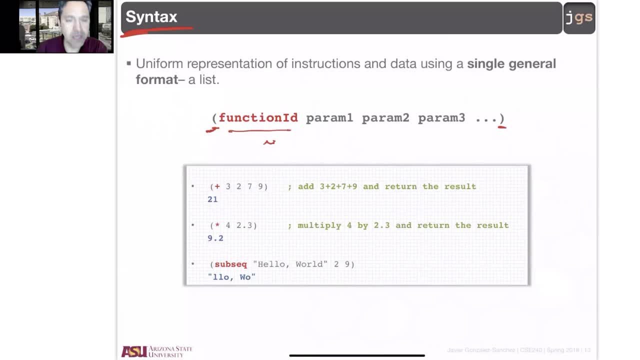 put the name of the action function that you want to run and you close your parenthesis- Anything that is after the name of the function and before closing the parenthesis, anything. they are parameters. So open parenthesis- name of the function- parameters. close the parenthesis. And very, very important. 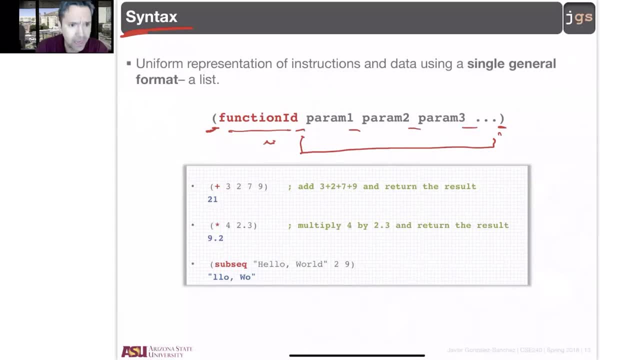 there are no commas, So examples: I want to do an addition. If you want to do an addition, then open parenthesis. I want to do plus an addition and I want to add two and two, closing parenthesis, That is. 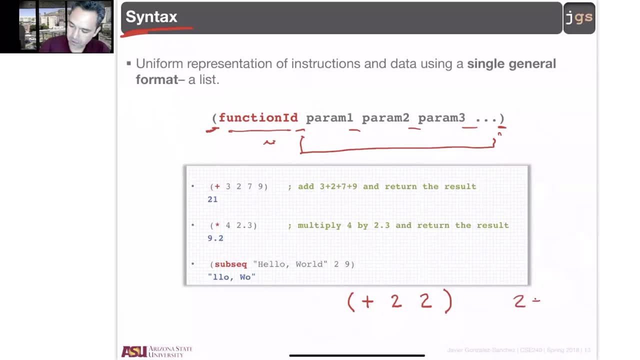 the equivalent of two plus two. in other languages The operators, even the binary, go first and then the operands as parameters. So you put plus two, two Okay, instead of 2 plus 2.. There is no operators in Lisp. Basically that plus is a symbol and is 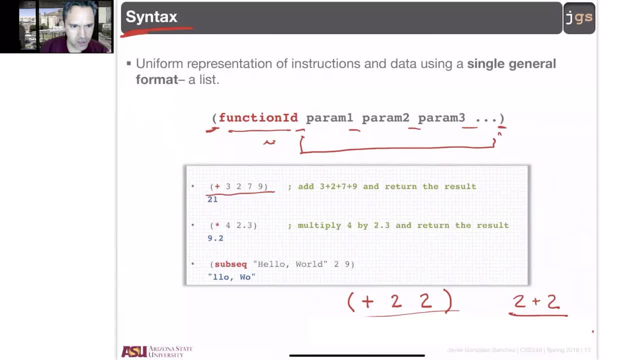 the symbol that is the name of a function, Usually in Java C and C++. plus is an operator and is a binary operator. Therefore, you do something like this, But if you want to do something like 2 plus 2 plus 3, you need to use two operators: Java C, C++ and the. 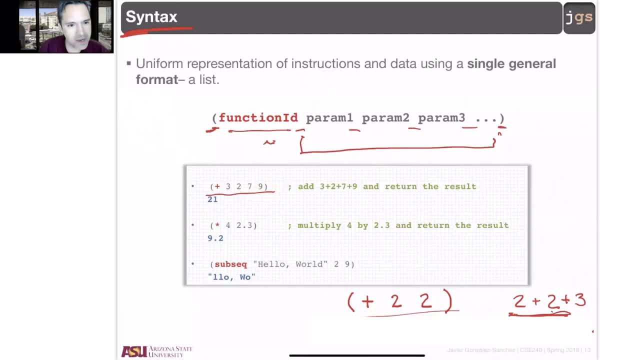 three numbers in Lisp, Because it's more like a function. what happens is, if you want to add several numbers- open parenthesis, closing parenthesis- the action that you want to do is the plus, and then you can put as many numbers as you want as parameters and the 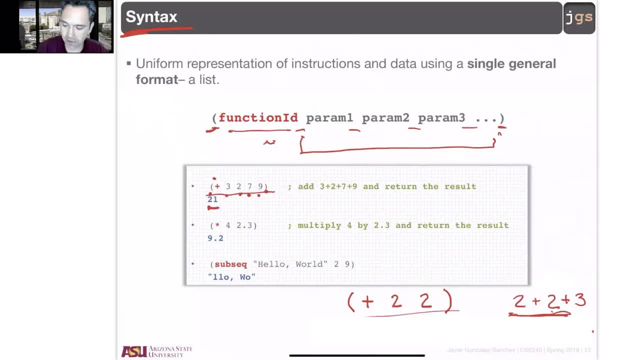 result is going to be this: The addition of all those numbers. So the result of this line is all this: Only one instruction, one action, The function ID, the plus, and you can have two parameters, three parameters, four parameters, as many parameters as you want. Similar action with: 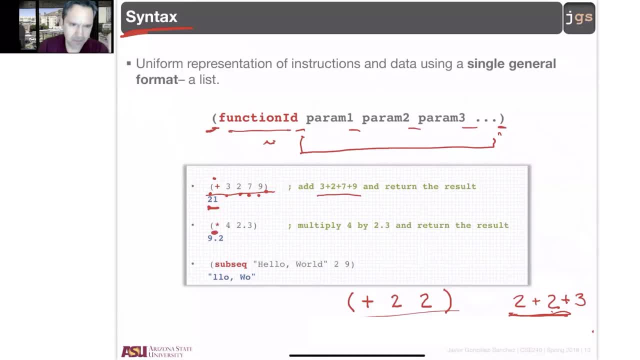 for instance, multiplication. Asterisk is multiplication, but in this case it's a function asterisk and you have one parameter, the four, and another parameter, 2.3.. You can have a function subseq- I am going to talk more about it- but this function 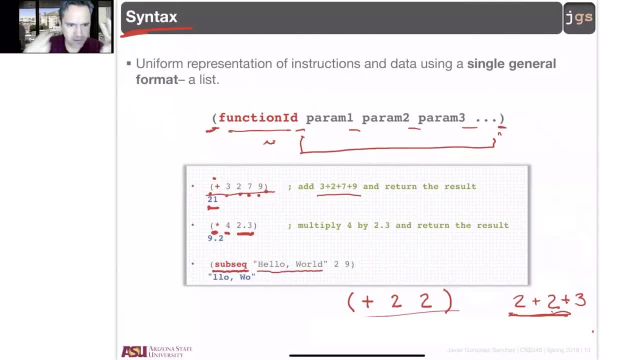 subseq receives one parameter, a string, still with the quotation mark, and two numbers, Three parameters. subseq is the name of the function. Very, very important. Every single function in Lisp returns a value. So let's see. 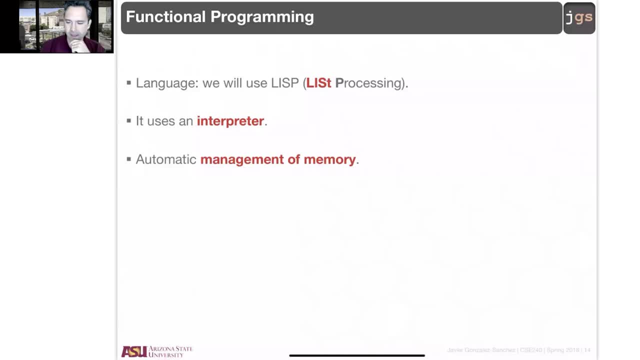 Let's see Lisp Key ideas. The name of Lisp means list processing. List processing Every single thing in Lisp: open parenthesis, function ID parameters. This is called a list. What is a list? Anything that has parenthesis open, parenthesis closed and things in between. 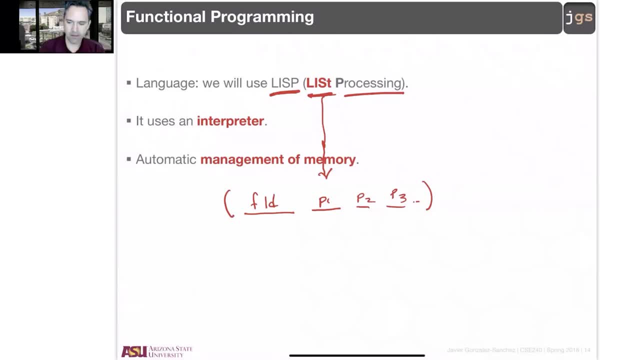 This is a list And processing basically is execution. You give me a list and I understand that in the list the first thing that you put is the action and the other things are the parameters and I am going to execute, run, process that list. If you put together, 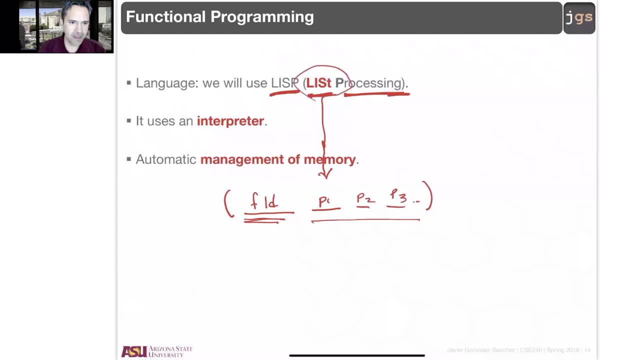 the letters. you play with them. you have Lisp, Lisp processing. Lisp works with an interpreter. Forget the compiler. Lisp only has the equivalent to the Java virtual machine. So you are going to use an interpreter for your Lisp programs. You have back the management of the memory. The interpreter is the one that is going to. be handling the memory. Now you have two things: One is the memory and the other is the computer. The computer is the one that is going to be handling the memory. The computer is the one that is going to be handling the memory. The computer is the one that is going 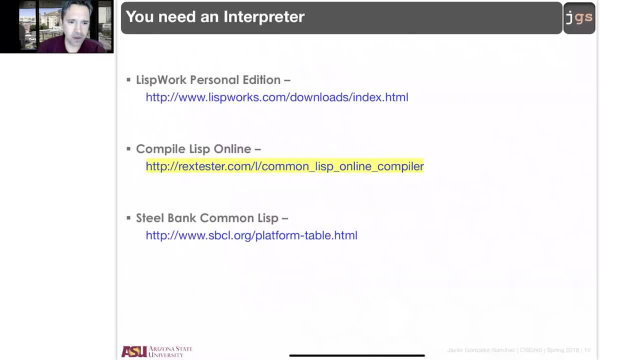 to be handling the memory. So you have two options in order to prepare yourself to start working with Lisp. Option number one: install the virtual machine in your computers. There are several options outside. I gave you these two links. In those links you can download the virtual machine and have the virtual machine in your computer. 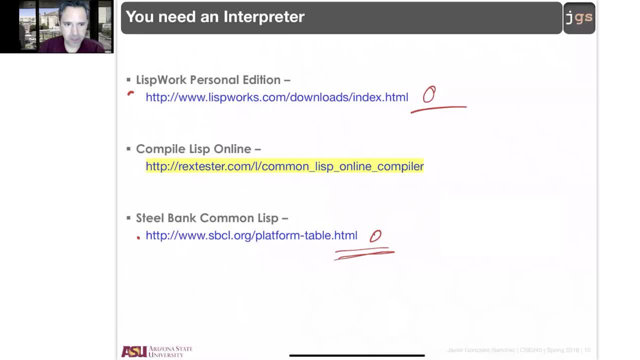 So that is an option. My recommendation, the option that I usually follow, is this one: So you do not need to install anything in your computers. Basically, you open a web browser, You open everything at any time, be it in practice, in your first. 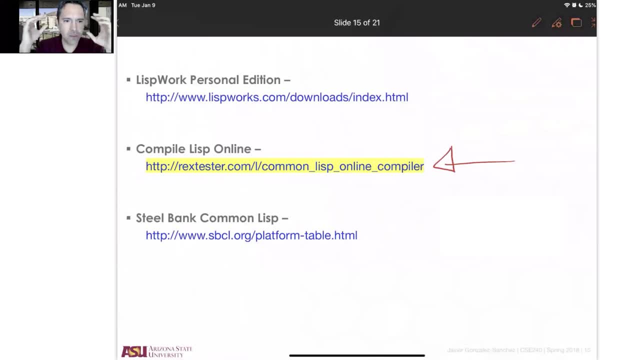 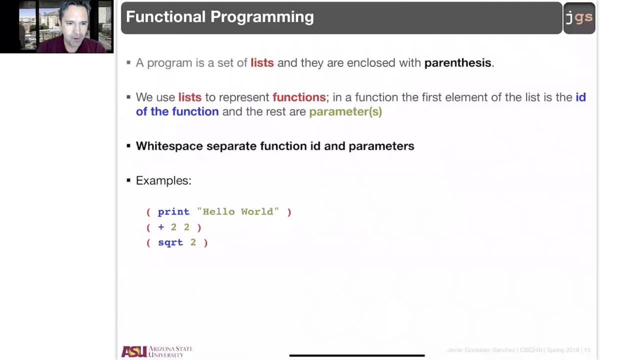 and inside of the web browser you have this screen in which you can put your program and you get the output of your program. So your program is executed in the server and the server show you the output. The hello world example in this, this is a program in this and with the thing that I described before, can you? 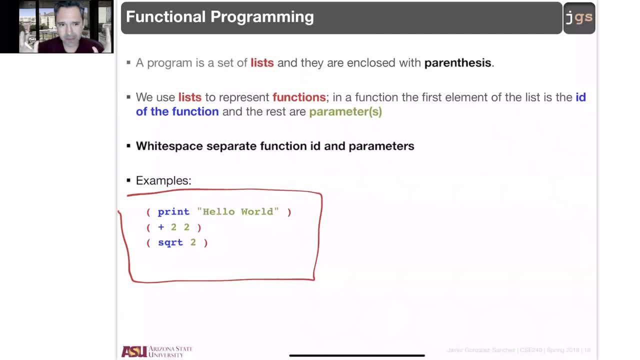 guess what is going to happen with this program that have three lines? What happened with the main? You do not need a main, That is a program, and the program have three lines. no main. Print is the replacement for system out. println in Java is the replacement of printf in C. is the replacement of cout in C++. 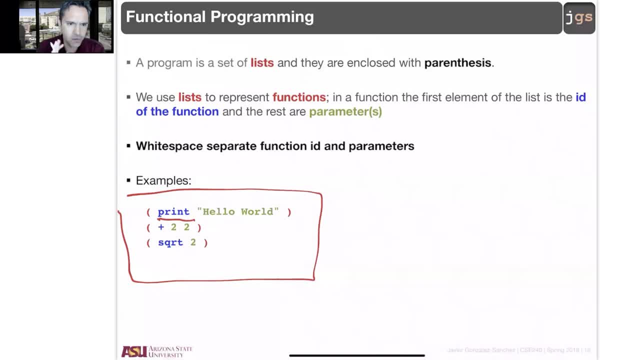 Use print. Print is going to print something in the screen. What, Hello world? the string Open parenthesis, closing parenthesis, no commas, no semicolon, nothing, Clean syntaxes. Second, I want to do 2 plus 2,. 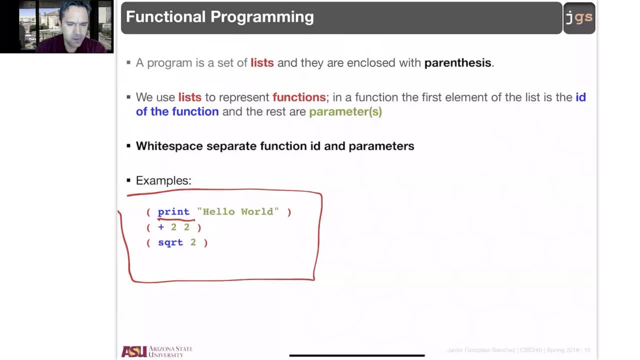 period. Last one: sqrt- Yes, square root. Use the same name that we use in the libraries in C and in C++ and even in Java. No need of mat dot something. Use the name of the action. The action is sqrt and one. 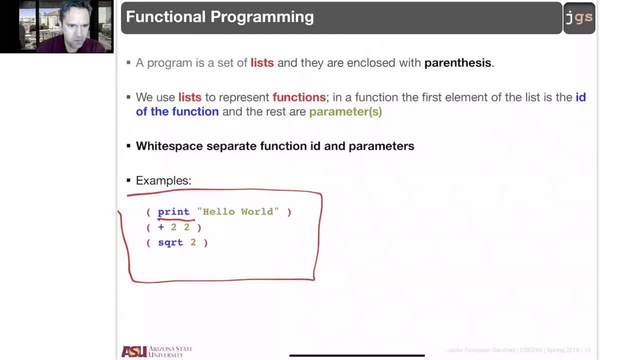 parameter the 2.. I want to make the square root of 2.. That's it Now. all the instructions, all the functions, all the list in Lispe. When you run the functions, every one of these is going to return something for the square root of 2. Is. 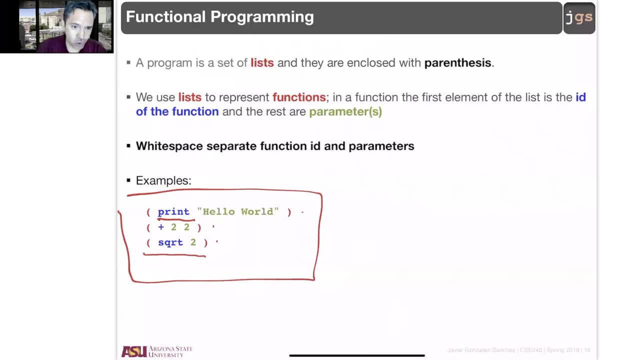 obvious. The return thing is going to be the results of the square root and healed of 2.. Let's say that чтобы votar con la mi hijita y voy a vender la misma root For the plus 2,, 2,. the return is obvious: It's going to be the result of the addition. 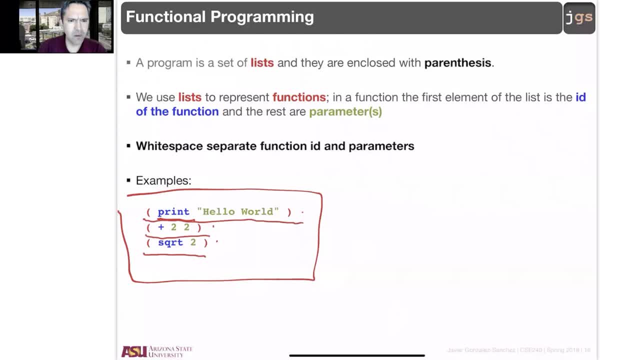 For this one, you can be thinking like what is going to be the return value of printing something? It's going to return something And the something that is going to return is the same thing that is printing. Remember, always, always, always, in Lisp, a function. 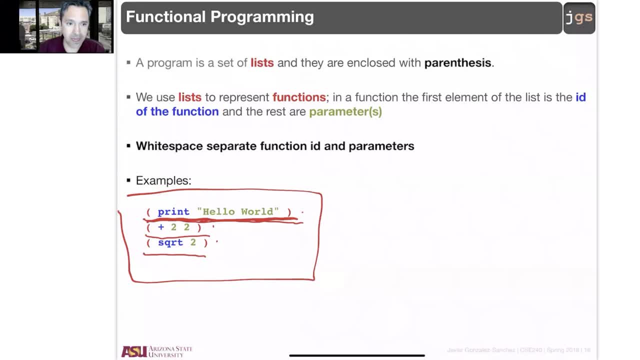 can return something, something Never bold, Never empty. So this one is going to print something on the screen and also return hello world. This one is going to return 4, and this one is going to return √2.. Everything that has parentheses…. 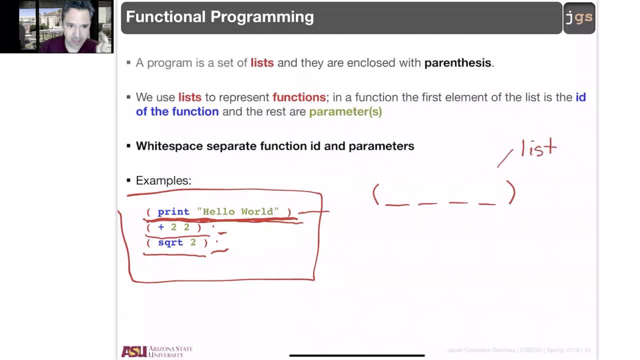 Something… something… something, something… is a list If in that list these first two element is a valid action id. this is called a function. again, anything inside parentheses with several elements inside this parentheses with things inside is a list. if the list have inside of the parentheses as a first element, a valid 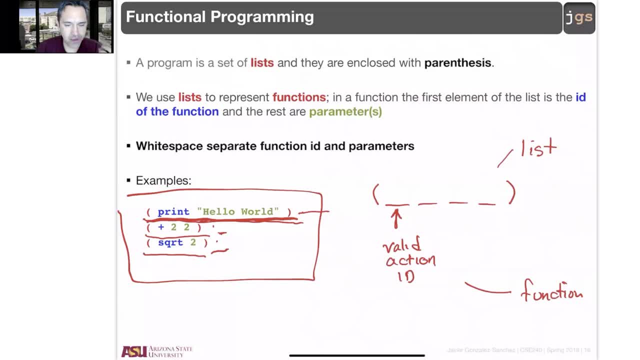 ID for an action, a valid name for a function that is called a function. a least is a function. yes, if the first element of the list is a valid ID for a function, how many least do I have in this example? so I have three lists. how many functions three? why? because I have three lists and all of them have as a 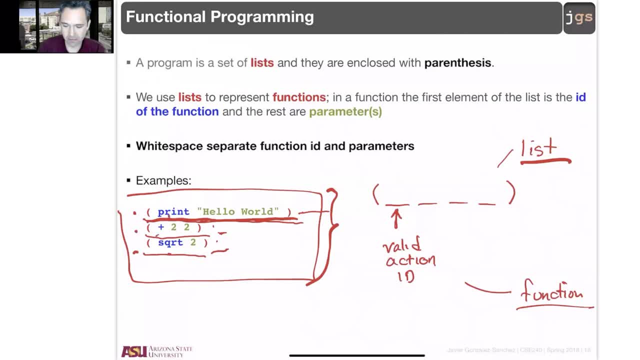 first element: a valid ID for an action operator, Matt printing. three functions. any function is a list, but not any list is a function. if you think about groups is like: these are the lists and these are the functions. any function is a list, but there are going to be lists that are not functions, because the first element is: 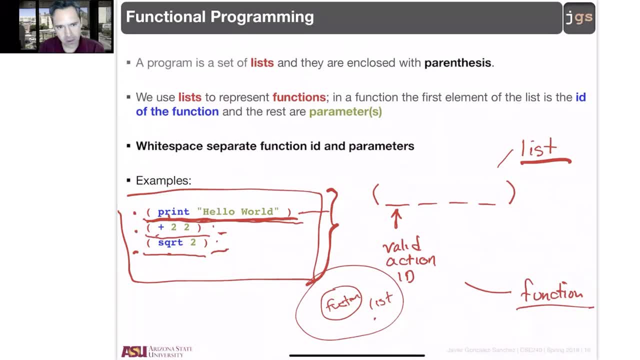 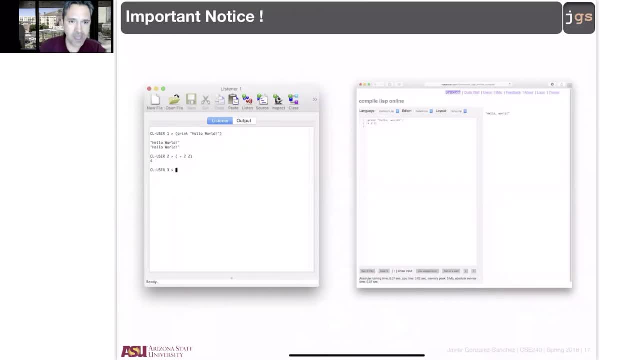 not a valid ID for an action. we're going to work with that later. so if you go and don't add any of the interpreters for lists of I mentioned before, you are going to have something like this, something that I want you to be aware. if you install locally in your computer an interpreter for this, it's. 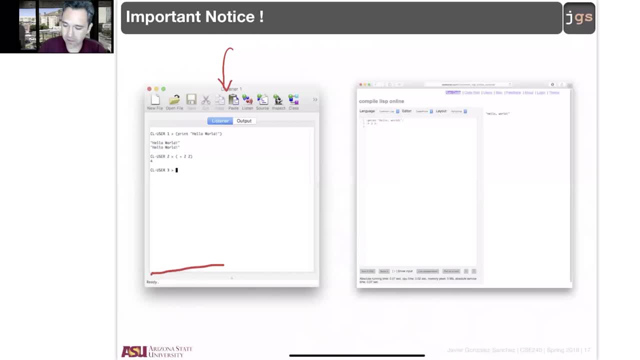 very, very, very simple. it's a window, a big window, in which you can start working with your program. basically, you put one line and immediately that line gives you results. You put another line and immediately that line gives you results, and so on. Every time that you close a parenthesis and press enter, you're going to get. 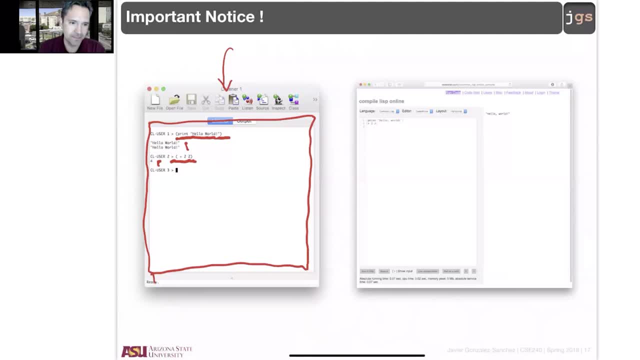 results Very, very important. Did you notice here, when you run plus two and two, you're going to notice the four. The four because that is the result of the function, So it's going to be printed, the four. Can you tell me why the print is? 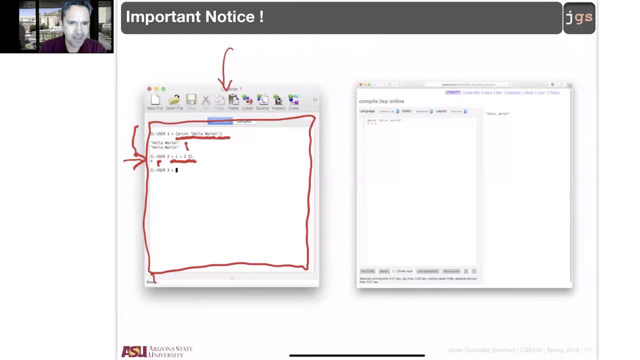 printing twice, hello world. Let me tell you this. The first one is the action of the function. The first one is the function is printing. therefore, the function is sending to the screen whatever you ask to send to the screen. The first one is because that is the result of the function. The first one is: 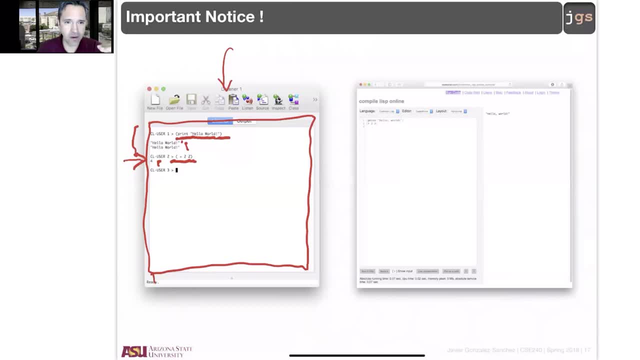 the action that the function is doing. The second one is because the virtual machine always, always, always show you the return value of the function and, if you remember, the print function returns the same thing that the function prints For this particular environment, local environment, is going to show you twice. 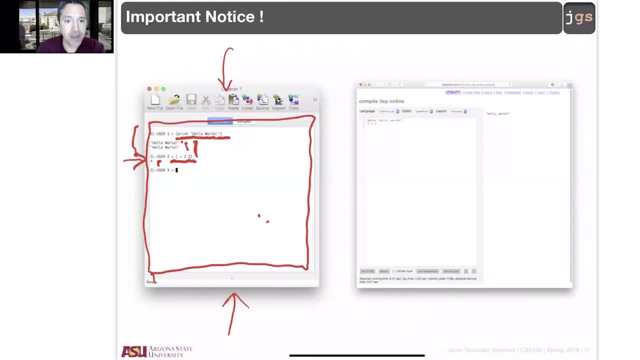 the result, One because is the action of the function and the other one because it's the return value of the function. If you notice, for the four you are looking: the four because the interpreter is showing you the return value of the function. In the second example here, if you use the one that you have online, 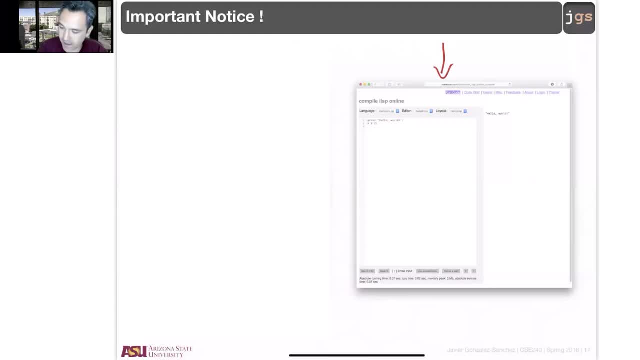 what usually happens with the online is you are going to have this space to create your program and the output instead of being in the same window, the online version. what they do is two different windows. This is my program. this is kind of the console with the output. Did you notice the difference? 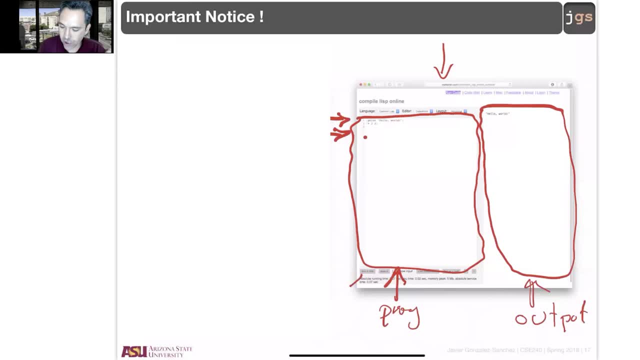 Everything together, two different windows. Press this run button here. Did you notice the output? The online one is not going to show you line by line the outputs. So if you want in the online to print the result of two plus two instead of just writing plus two and two, 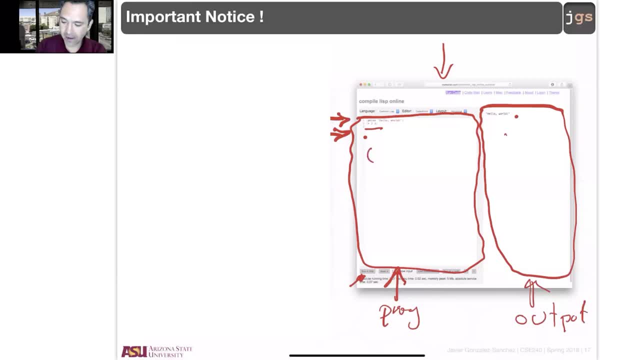 you need to ask for that to be printed, as we described before. If you put this line there, then you are going to have the four in the output. So the correct program, the good one, is this one: Printing in the output only if you ask. 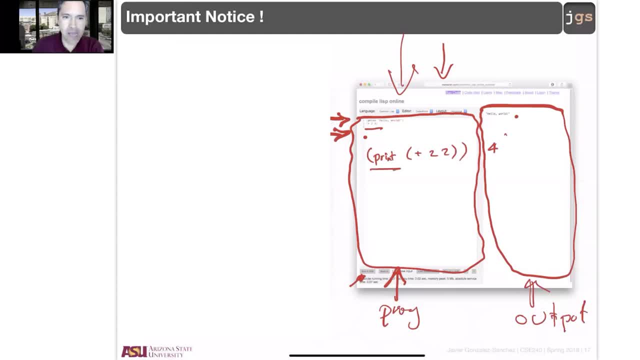 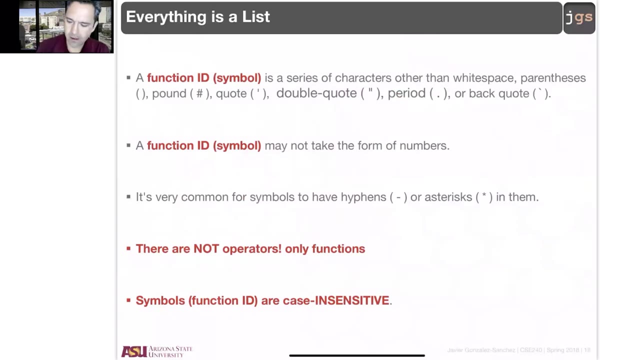 something to be printed. That is what you do with Java, That is what you do with C, C++. If you want something in the output, you ask for that something to be printed. Moving forward Rules, A function ID could be remember. the function ID is the. 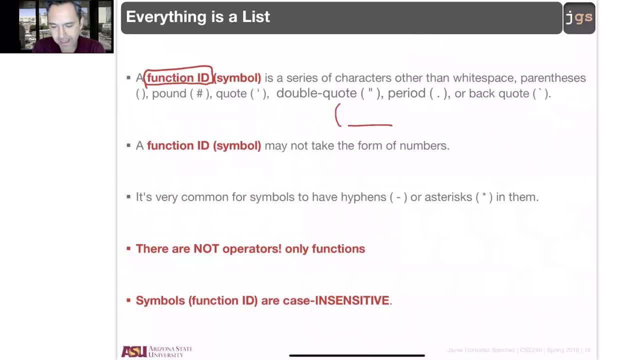 first thing that you put after opening the parentheses. The first thing that you put after you open the parentheses can be almost the same as the first thing. that is the name in the output. That is the name in the output. It can be the last of the. 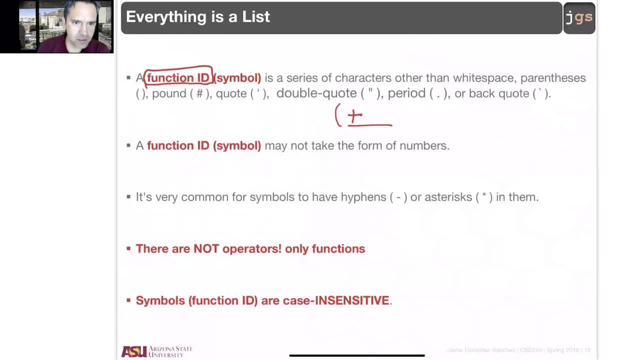 names in the output. It can be anything. It can be like before the plus, it can be like before the asterisk, or it can be a name like SQRT or print. Whatever you put as a first element after opening the parentheses is going to be considered like the function ID. 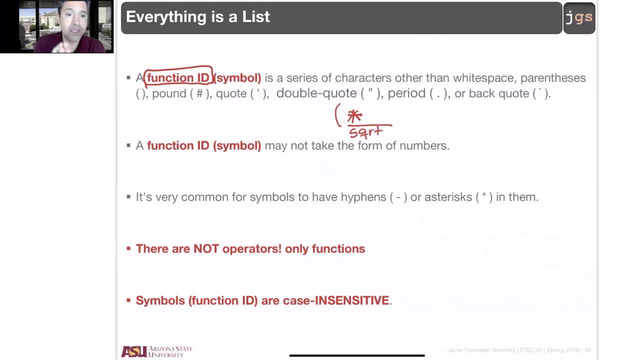 Now, the only thing that is used to separate the name from the parameters is the way that you put a function ID to the output parameter. We will talk about the second thing in the the white space. So if you put something like asterisk, x, y, c, because there is no, 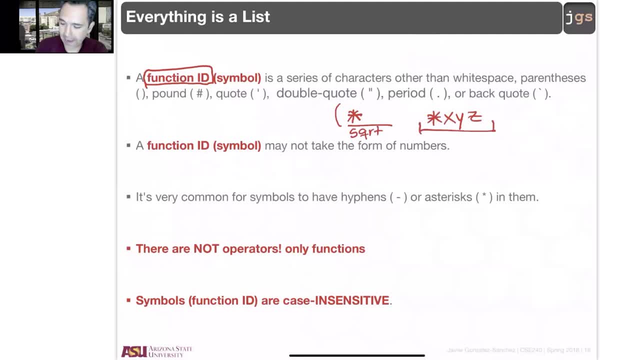 white spaces for the interpreter: asterisk, a, y, c minus one. all that is kind of the name of the function. It's the name of the function that you want to use. This minus is not an operator. This one is not a number, All these things, whatever you create for. 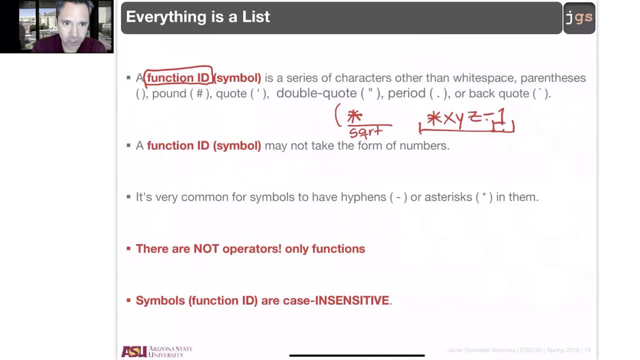 the interpreter is the name of the function that you want to run. Similar if you open parentheses plus space plus. this plus is the name of the function and this plus is going to be considered the first parameter, which is different from plus plus together. 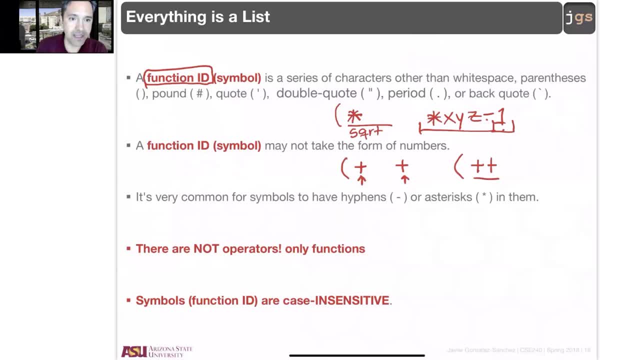 without the space, Plus plus together is going to be considered the name of the function, the name of the operation that you want to use. So the most important, and only the limited in Lisp is the space, The white space. The white space is the one that is going to help you to separate functions and parameters. 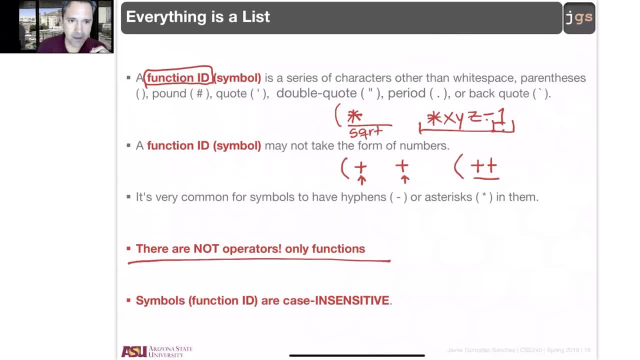 Not a comma, No commas here. Oh, not yet No operators in Lisp: The plus, the asterisk and so on. they are functions, Yes, with the same symbol that the operators in Java, C, C++. but they are not operators, They are functions. The correct name for them is functions. 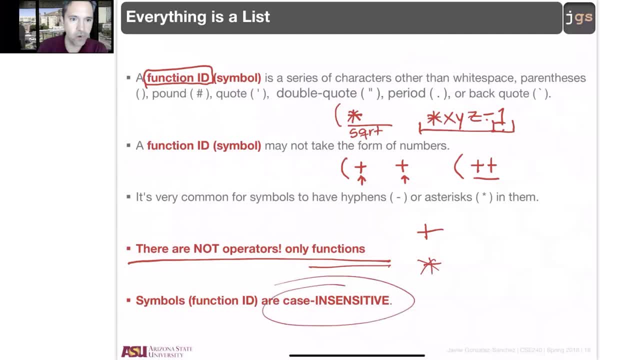 But that is not Lisp, But a key idea. with Lisp You can forget about the difference between uppercases and lower cases, so you can do open parentheses Print, or you can do open parentheses Print, or you can do, as I before, everything lowercase print, and those three are the same Lisp do. 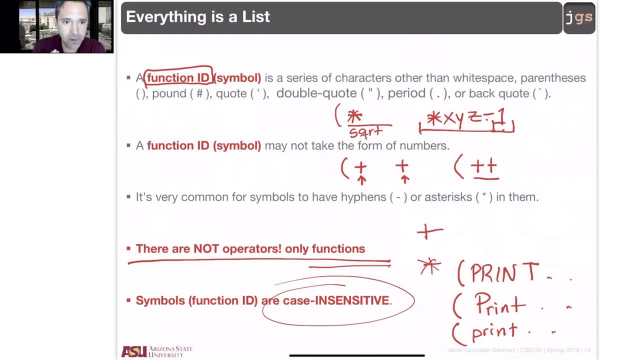 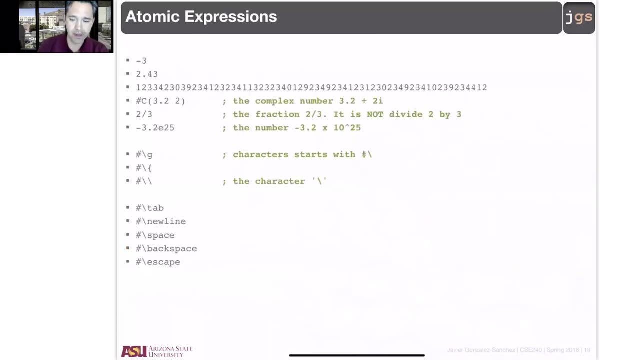 not care about upper and lower case. Sorry, lower cases. you can call print the function everything uppercase, you can call print the function everything lowercase and you can make a combination of upper and lower cases and they are the same. so this is regarding the instructions. now, what about the parameters? and for the parameters, number? 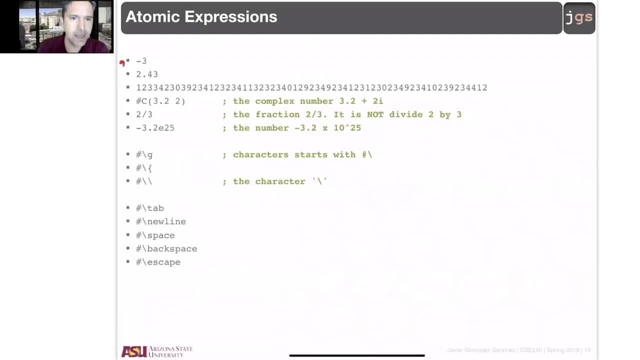 one, this guy here minus three. so in lisp that change. in lisp the minus here is not an operator. the minus is part of the word this guy is one word in lisp. therefore, if I do plus three, minus two, you need to be very careful because this minus two is not an operator: minus. 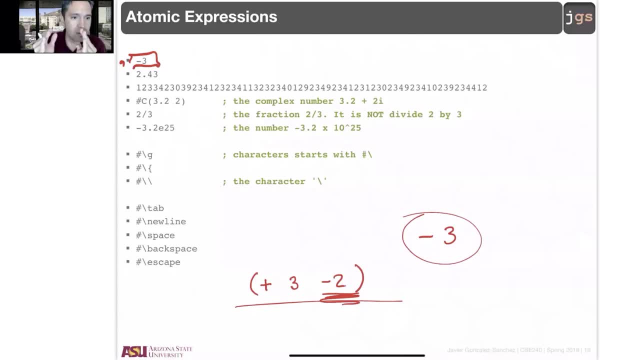 this minus two together is one word, one parameter, and represent the negative. two makes sense. if that was a, if that, if that was a parameter, would it be put it right after the plus. it's the same. I mean this one is kind of three plus minus two and you can put it right after the plus and you can put it right after. 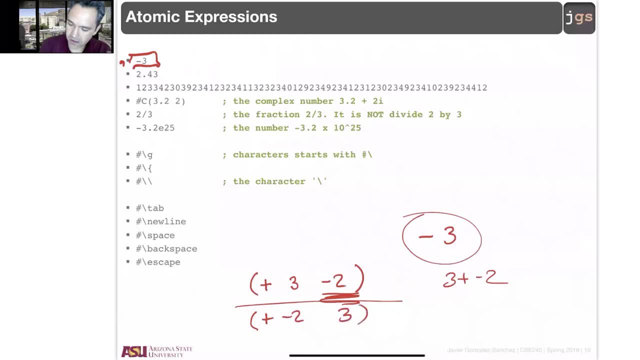 the plus, and you can do plus, minus, two, three. the only thing that we need to be careful is white space here, separating these two elements. what white space here? and you are going to have this idea of minus two, plus three. that is basically the meaning. the only thing that I want to be sure is when you look at this: 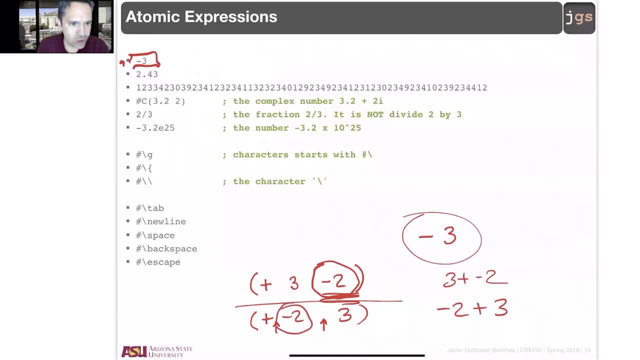 minus here. minus here they are one word. second, these guys, the floating point numbers and so on. they exist in lisp. next, what do you think about this line number three? it's an integer right, a lot of numbers together. one integer- if you use that one in Java, C and C++- is an. 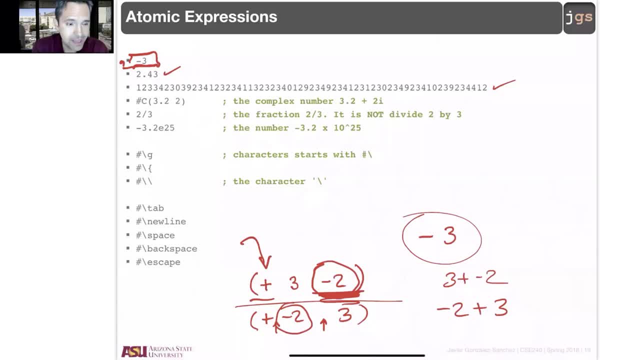 error. it's an error because it's too big. that number in lisp is an integer and is valid, is correct, is fine. in lisp you can have long, big integers and they work. complex numbers in lisp, you have complex numbers and this is one word. this is one word. this represents one number and the 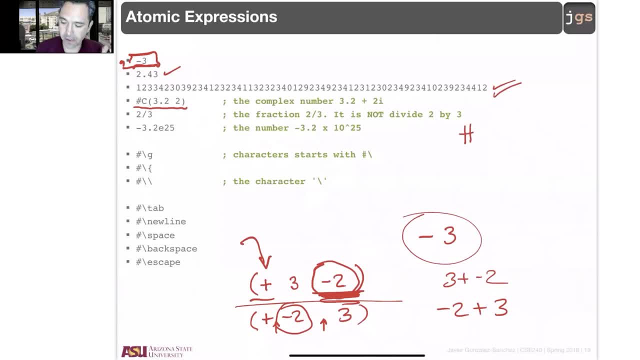 syntax is is basically sharp C parentheses. again is the only place in which you use parentheses not for a list but as part of creating one element, and inside you put the real part, a space, not comma space, the imaginary part. so in this case this is the complex number three, point two: 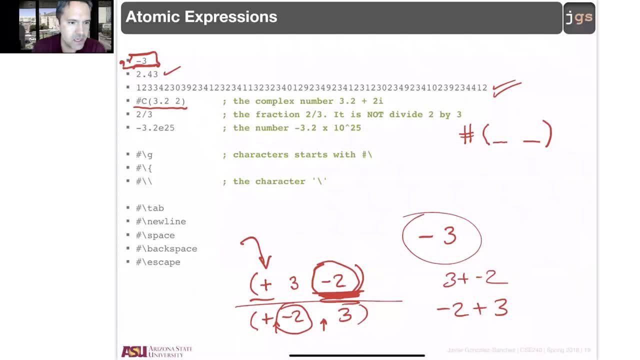 real part plus two, the imaginary part. good, okay, I need to explain what is the meaning of this. if you remember the backslash, backslash comments in Java, comments in C, comments in C++, they have been always, always, always this backslash, the comments in lisp, I think you figure out now what is. 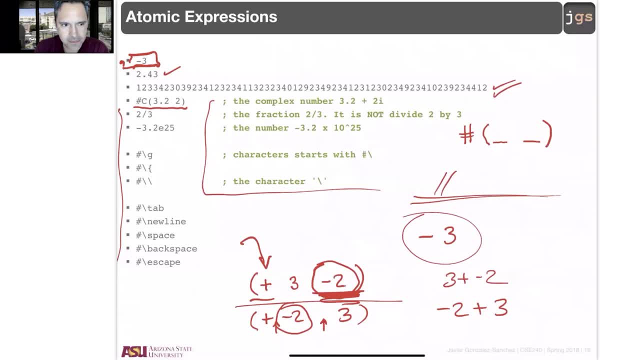 the character that we're going to use to open a comment in lisp: the semicolon, so no semicolons at the end of the line. now the semicolon is the one that is going to start a comment. so here I do not have comments. here I do not have comments, and. 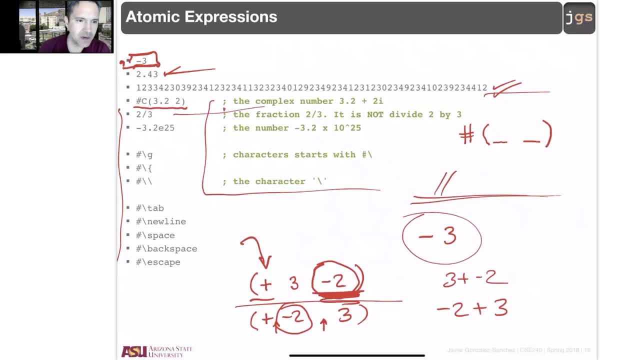 here. if I put a semicolon at the end, what I am telling is: okay, this semicolon is open in a comment. Good, This one. in Lisp we have fractions. So this one two, division three is not a division. That diagonal is not a division operator. That one, those three. 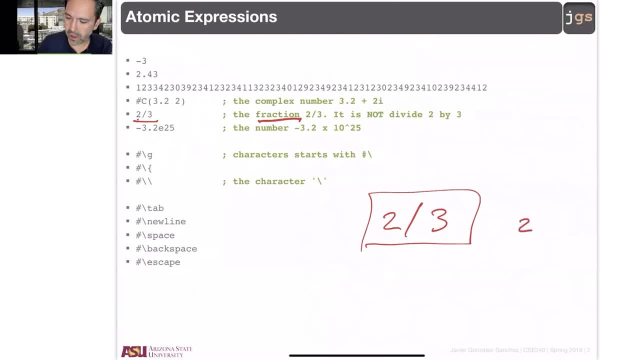 characters together is what we usually know, like this fraction. We have fractional numbers in Lisp and they are going to be represented, used like we usually represent division in other languages. But very, very important. If I want to do a division, what I need to 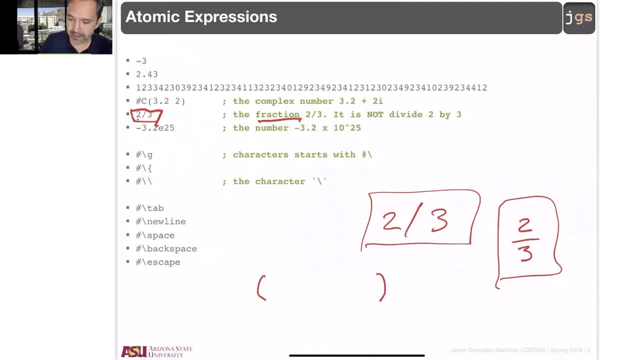 do is open parenthesis, close in parenthesis. the function ID is going to be like the division ID. This is the division operator that we have before, and I can do the division of whatever I want. This is a division operation, But if I have this, this is a number, This is: 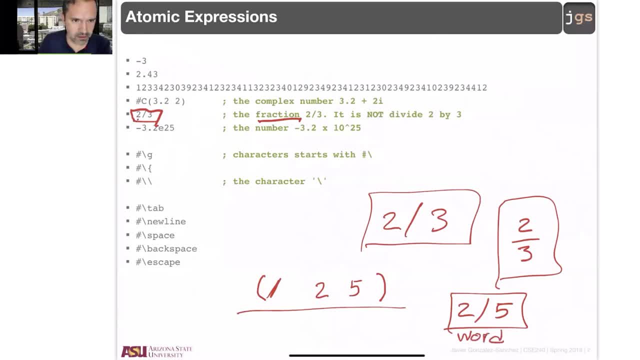 one word, Not an operation. Obviously, if you do the division of this, the result is going to be something like this. So Lisp is going to tell you the result of dividing two slash five is going to be the fraction two slash five. 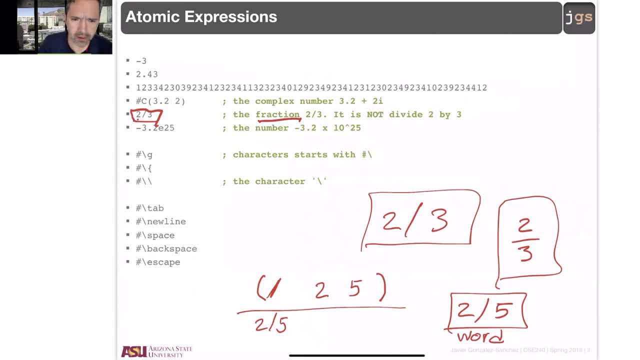 Now, obviously, we can use the notation with the I, this notation, or use the dot, whatever we want. This is everything regarding numbers, New things, the negative, the fraction and the complex. Very important thing. Now for the characters, usually in Java, C and C++. 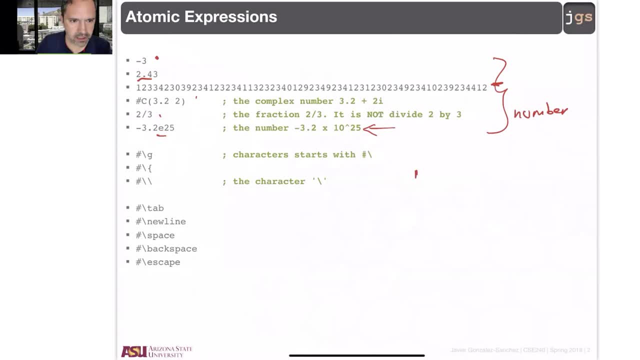 when we talk about division, we are going to talk about division, We are going to talk about characters. It was like single quotation mark, something. single quotation mark. This was the lexical rule for the characters in C, C++ and Java. One exception: two characters. 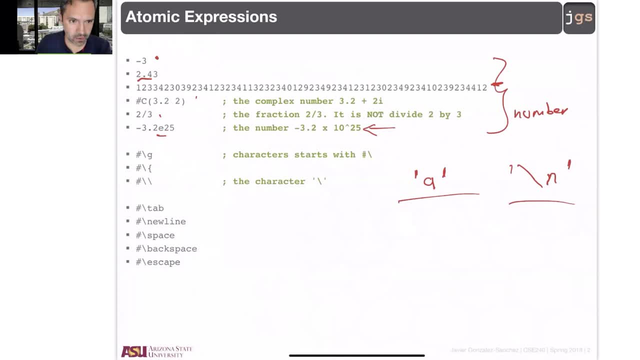 inside of the single quotation marks for the escape sequence: Backslash n, backslash t and so on. In Lisp, instead of using the single quotation marks, a character is going to be something that starts with a sharp and backslash. These two guys are the replacement of the. 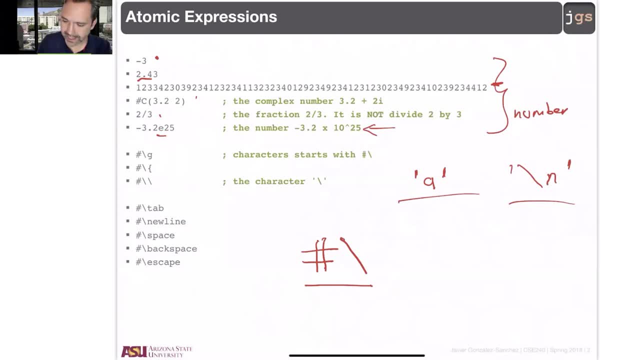 quotation, single quotation marks. So, for instance, this one, the character A, is going to become this. So, if you notice, this is the character, this is the character, and what we did before was to put the single quotation marks right and left. 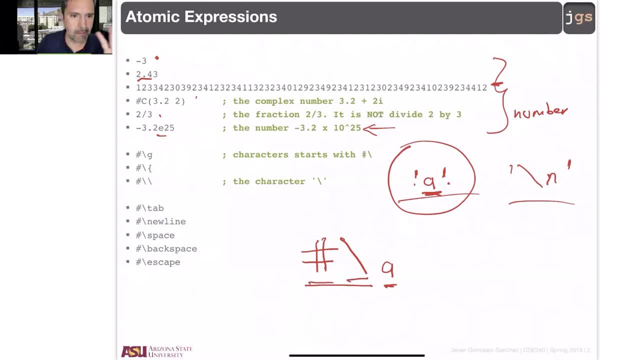 Now we put sharp and backslash, Similar to what we did before. if we want the character backslash, we put that one twice. So this is because the character and this one is the character that we want. What happened with the backslash n or the backslash t? 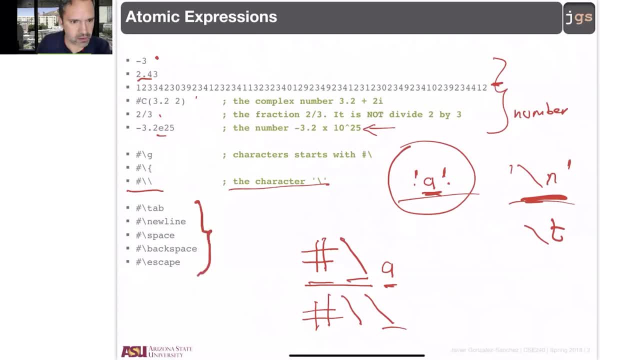 and so on. You can notice something that is going to happen in Lisp is no more backslash n. In Lisp it's going to be yes, sharp, yes, backslash, but now, instead of using the n, we use the full name new line or we use the full name tab or space, instead of using 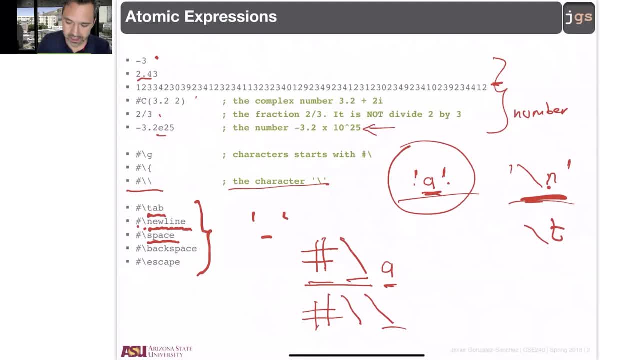 this, this and one space here. This is the character for space, Backspace, so the back key. instead of this we can put the full name Escape. The key escape is this character. So now we use the names Very, very important. 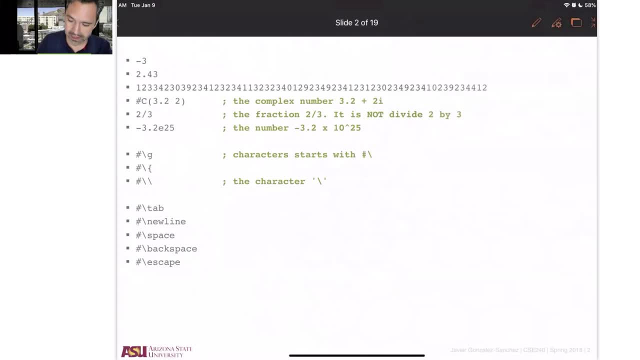 Those, even though they are words. all of this is one character, is the value for one character and the same here. So the rule, instead of the single quotation marks: sharp, sharp backslash, and then whatever you put in size here, now it's going to be here. 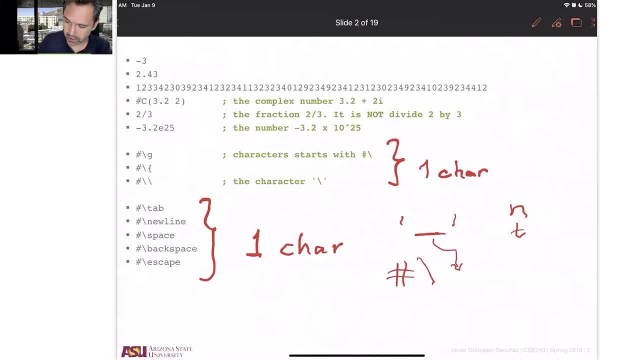 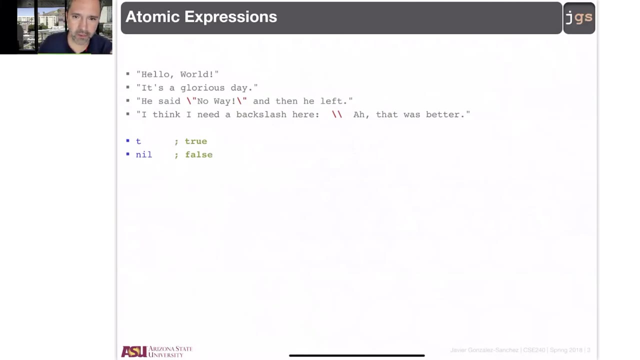 And now, instead of the n or t and so on, with the backslash, now we have particular words. So numbers, characters. What about the strings In Lisp? strings as usual, quote inside whatever you want, and this one is one element, one atomic element, a string value, Same one. 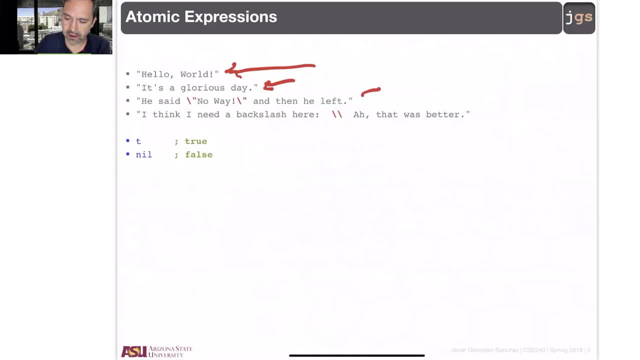 here And, as usual, if you want to use the quotation marks inside of the string, you can use the backslash to tell the computer: hey, this quotation mark is not crossing the string, but I want the quotation mark inside of my string. This is exactly the same thing. So I just put a string lower. This is exactly the same thing. So whenever we use quotation marks inside, we have to look at the string, We have to look at the string and we have to look at the quotation mark, And this because the quotation mark is not closing a string.